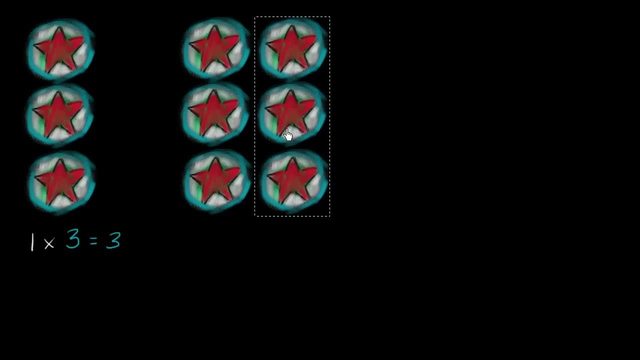 So that's one group, and then here's a second group, Here's two groups of three. So how many total star patches do I have now? Well, I have two groups of three. Or another way of thinking about it is: this is 3 plus 3.. 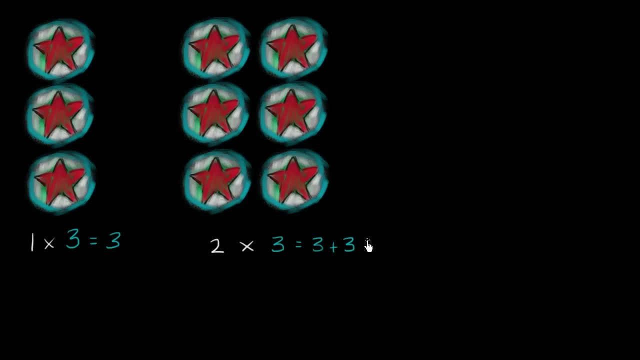 This is equal to 3 plus 3,, which is equal to 6.. So we see 1 times 3.. One group of three is 3.. Two groups of three, which is literally two 3's is 6.. 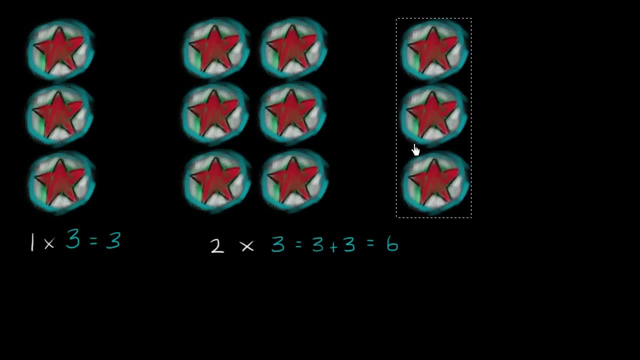 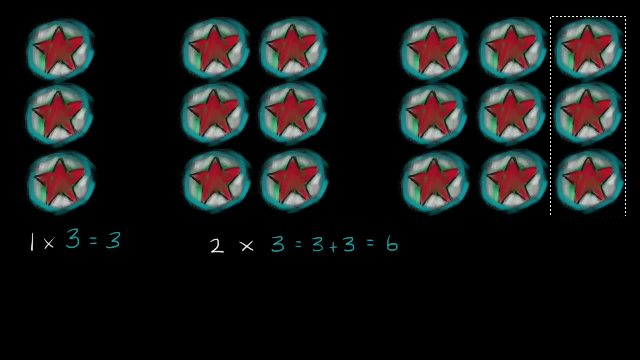 Let's make it even more interesting. Let's have three groups of three. Three groups of three. Now, what is this going to be equal to? Well, it's three groups of three, So I could write this as three groups 3 times 3.. 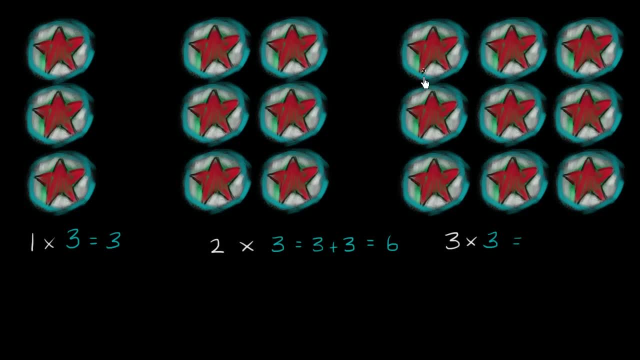 And how many of these star patches do I now have? Well, this is going to be 3 plus 3 plus 3.. It's going to be 3.. 3 plus 3 plus 3.. Notice, I have three 3's. 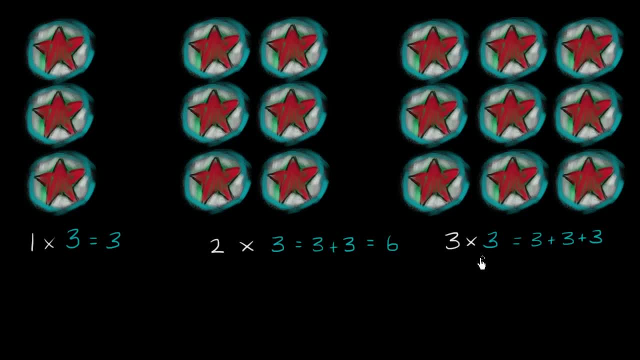 I have two 3's, I have one 3.. So this is 3 plus 3, plus 3 is equal to 9.. And you can count them: 1,, 2,, 3,, 4,, 5, 6,, 7,, 8,, 9.. 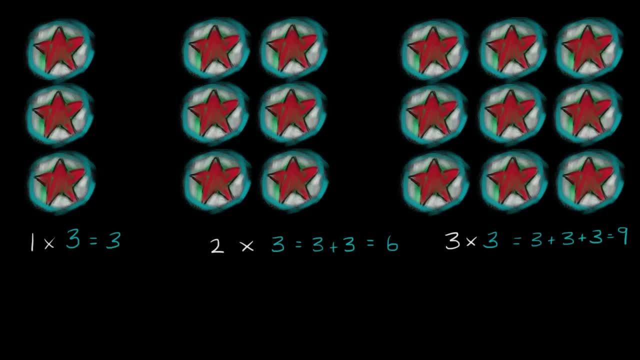 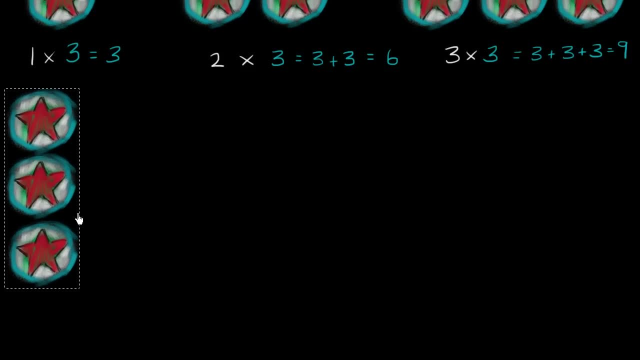 Or you could just count by 3's, 3,, 6,, 9.. And I think you see where this is going. Let's keep incrementing it. Let's get four groups of three. So let's think about what 4 times 3 is. 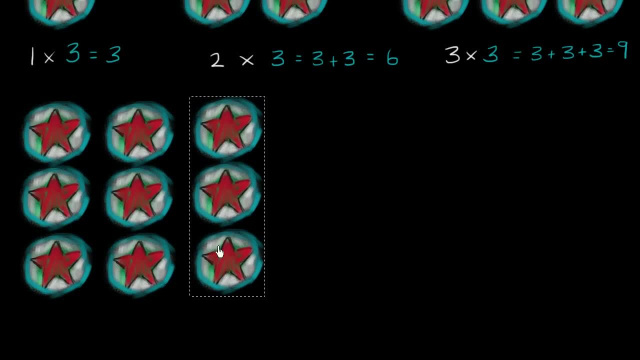 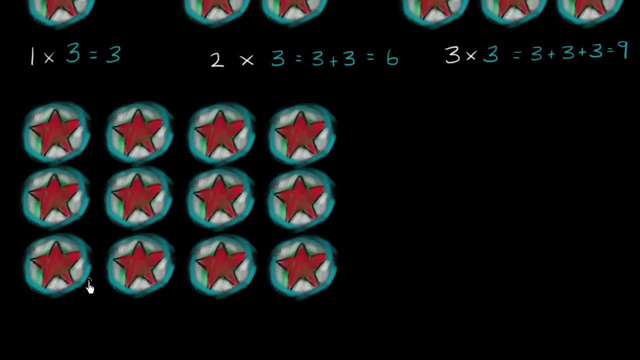 1,, 2,, 3, and 4.. This right over here is four groups of three. We could write this down as 4 times 3, which is the same thing as 3 plus 3 plus 3 plus 3.. 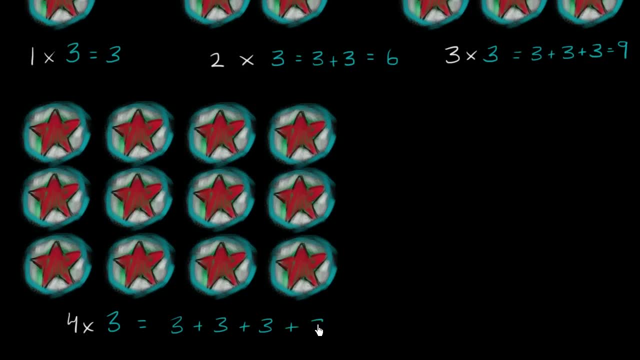 3 plus 3 plus 3 plus 3.. Notice, I have four 3's, One, 3, two, 3's, Three, 3's, four 3's, One, 3,, two, 3's, three, 3's, four, 3's.